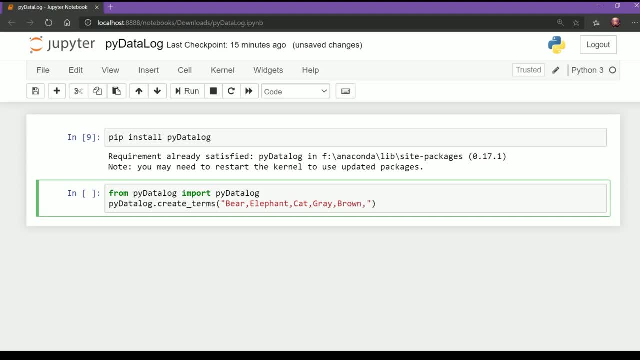 So PyDataLog has an inbuilt function known as create terms, where we create all the terms which belong to the facts and rules. So here we create: bear, elephant, cat, gray, brown, big, small size, as well as color and x, I'll say y, x is used and dark Yeah. So let me now define. 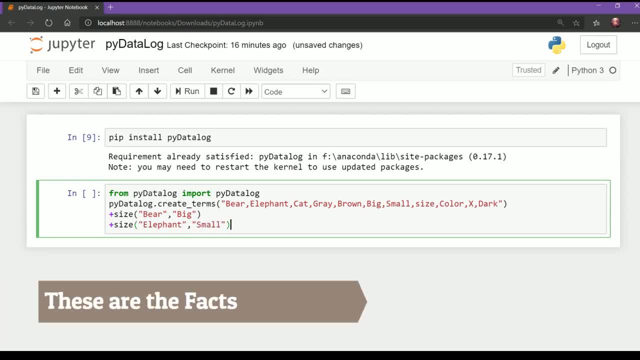 all the given relation. So here, this relation, we will read this relation, as bear is big, elephant is small, learner is big, andily meter is, I believe, is two большой and paper his. So in this case we can write out random numbers and other groceries and bags or things like that. 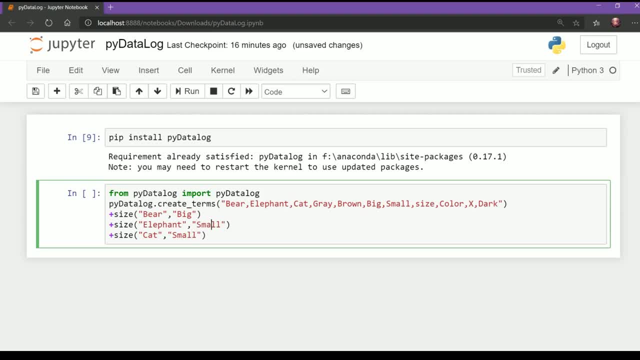 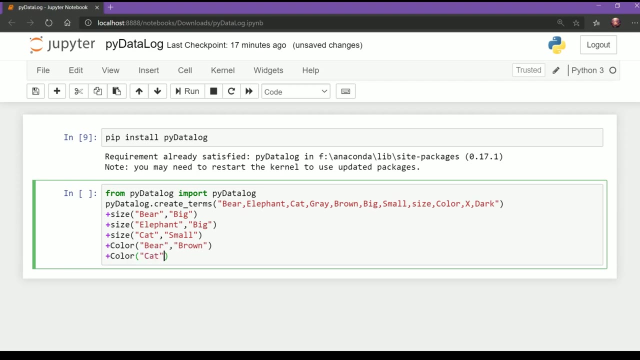 We can also write up the relevant activationogy. So let's get prepared for a call. and Mercedes, Yeah. So let me now define all the given relation. So here, this relation, we will read this relation, as bear is big, human is big, cat is small, and so on. 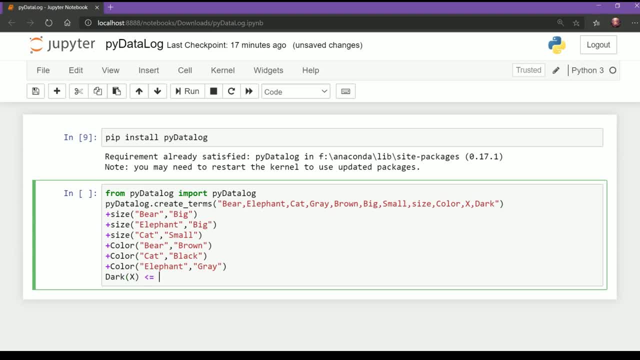 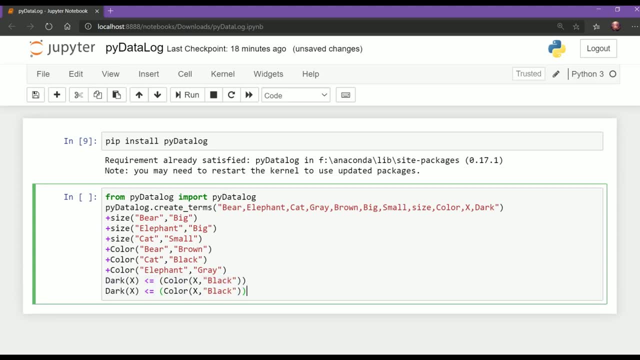 so now here i am declaring relation dark of x, that is, if x is an animal, it is called dark if its color is black or brown. so in our question we need to print an animal which is dark and the size of the animal should be big. so print dark of x and size of x should be big. so here 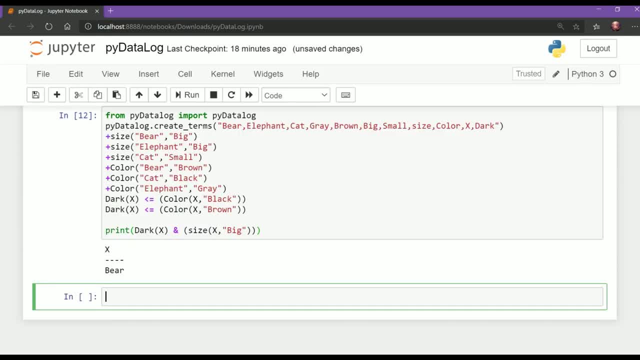 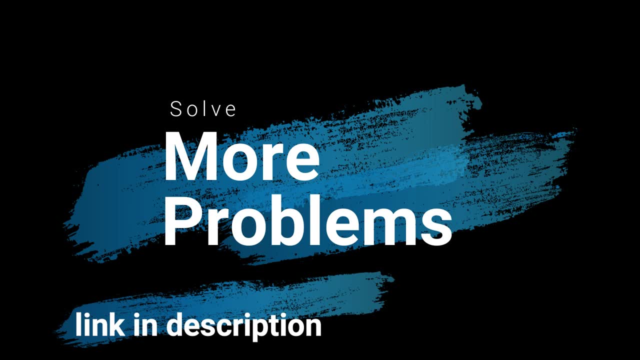 we get bear as the animal which has size, big and the color is dark. so if you want to solve more problems in computer, you can use this problem. so here we get bear as the animal by data log. the problem link is in the below description and the solution is also provided. 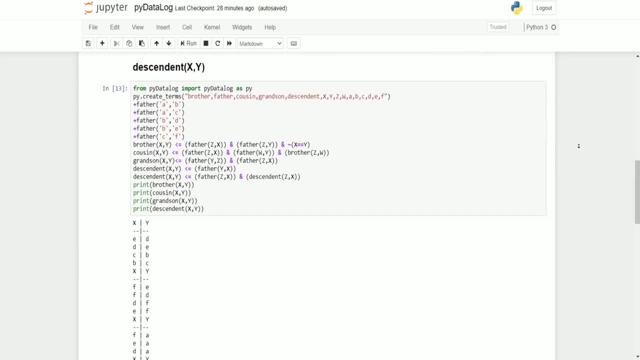 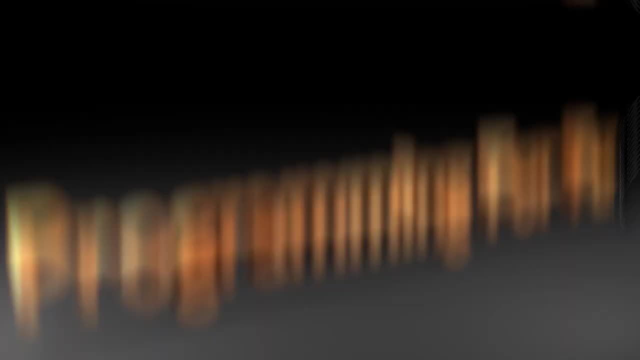 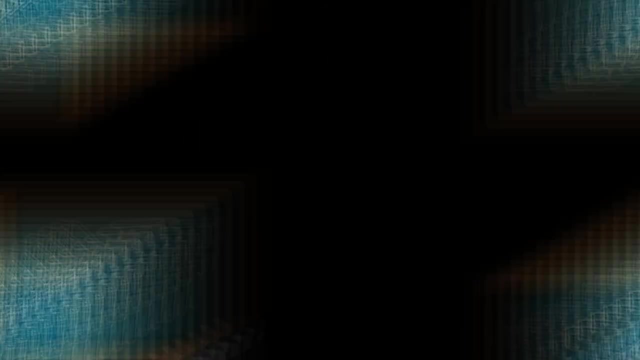 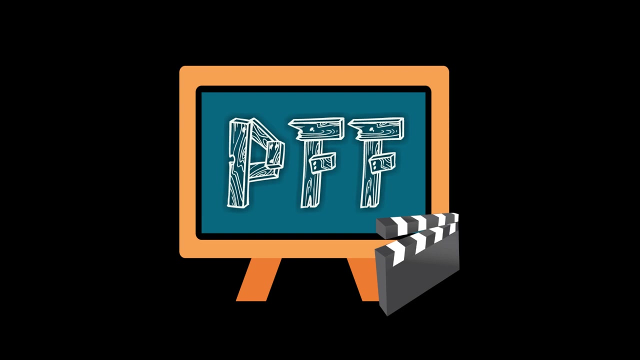 with that, subscribe and stay tuned for more updates. thank you and good bye you.